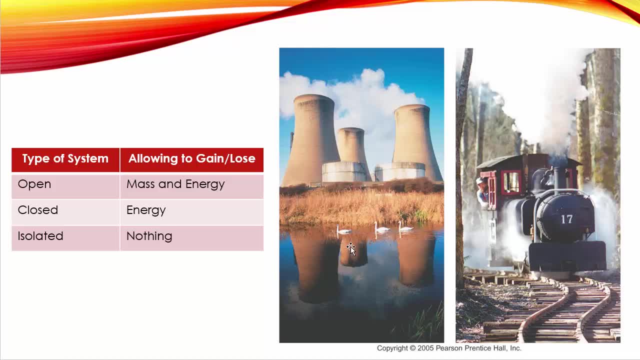 And in all those situations we are harvesting heat for its energy, which is a very inefficient thing to do, but there tends to be a lot of heat around, so it can be a quite useful thing to do. So we're going to now look at some more complex processes rather than just: PV equals NRT and Q equals MC, delta T. 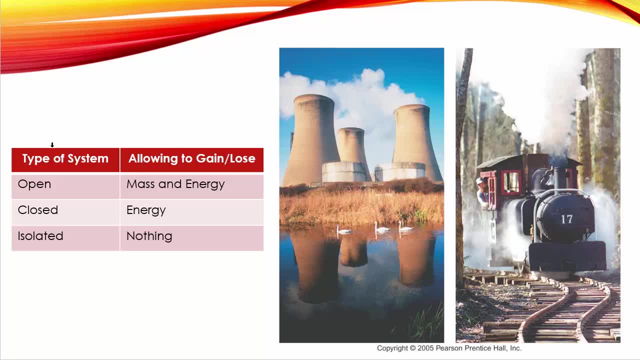 Before we get into it, just a little bit of terminology. I think I've gone over this at one point or another. but we have different types of systems and ways that we define them. An open system: We can gain or lose mass and energy, so it's really not a system at all. 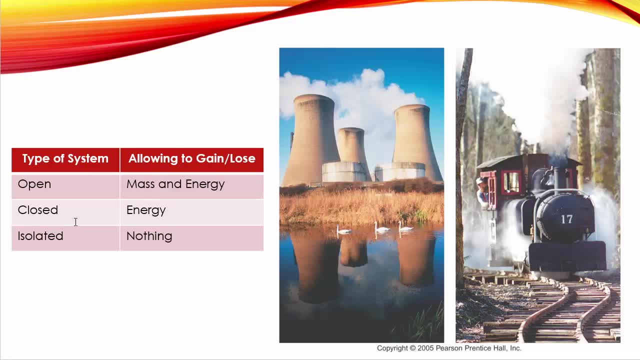 It's just free for all. Anything can come and go. A closed system is one where we still allow energy to go in or out, And most of these thermodynamic processes we're going to look at are what you would call the closed system. 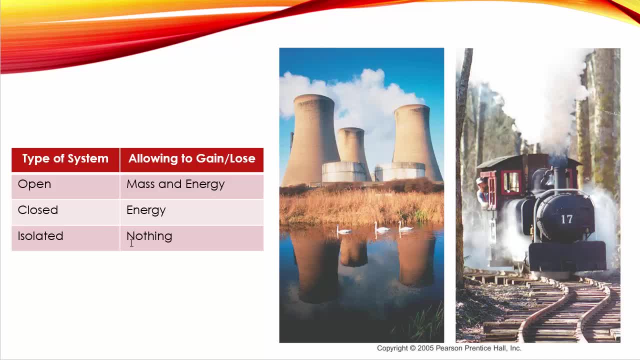 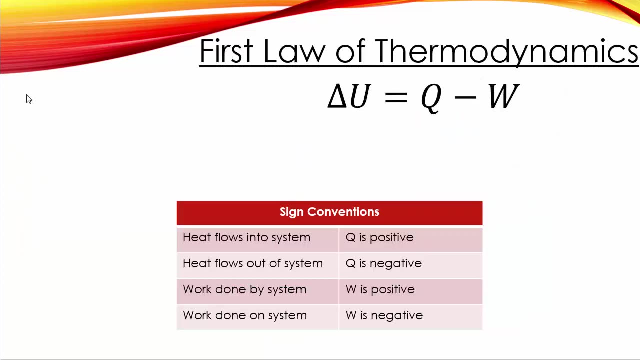 There is, in addition to that, what's called an isolated system, where you can't exchange matter or energy. A lot of times people call an isolated system a closed system, But they mean isolated. Anyway, moving right along, The first law of thermodynamics, which was developed before we had a full understanding of the law of conservation of energy, 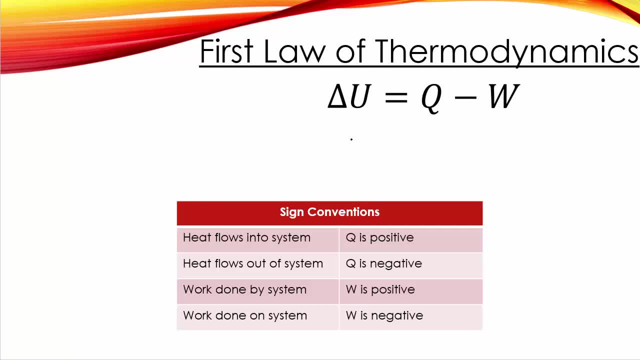 says delta U equals Q minus W. Now this U we've already encountered. That is what we call the internal or thermal energy. Internal energy Q we've already encountered as well, That is the heat flow- And W- we haven't really used that in a thermodynamic context yet. 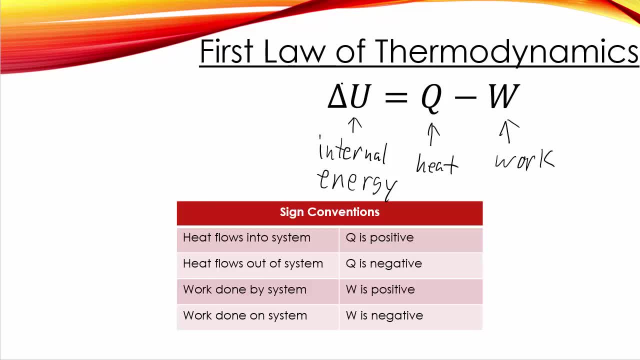 But that is our old friend work. Now, this equation here is known as the first law of thermodynamics, And it's just a statement of conservation of energy. So if you have a gas or some other thermodynamic system, the internal energy of that system, if it changes. 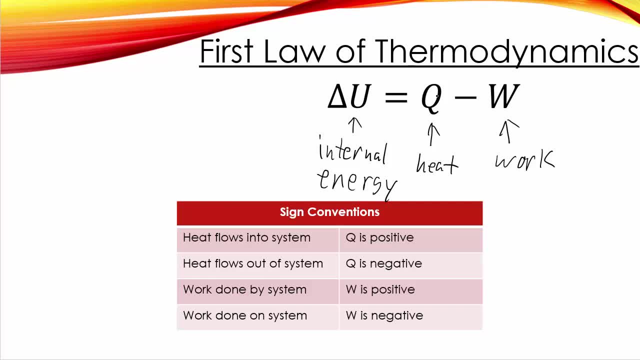 the changes will equal how much heat Went into or out of the system And how much work was done on or by the system, And I'll go over some more examples that will make a little more sense. You do need to be careful about the sign convention of these things. 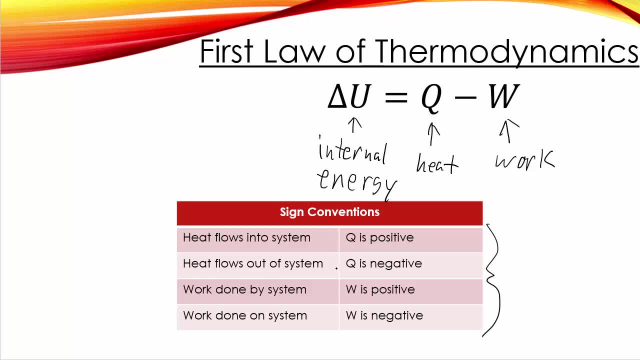 If we say that heat is flowing in, then Q is positive. Heat is flowing out, then it's negative If it's work done by the system. So, for instance, we're going to have a lot of situations where we're just thinking about a piston. 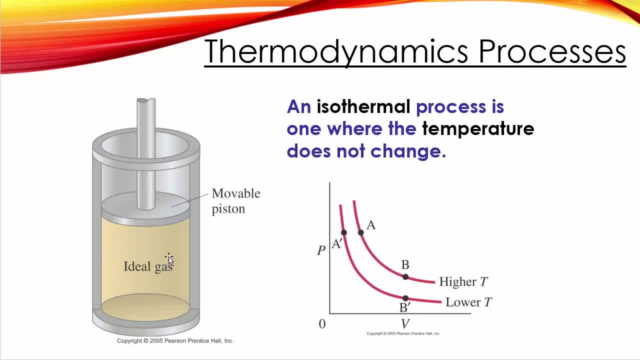 And a gas. This is what happens inside the engine of your car. So if that gas is pushing on the piston And then that goes through a drive train and makes your wheels turn, Then the gas is doing work. So we would say that's work done by the system. 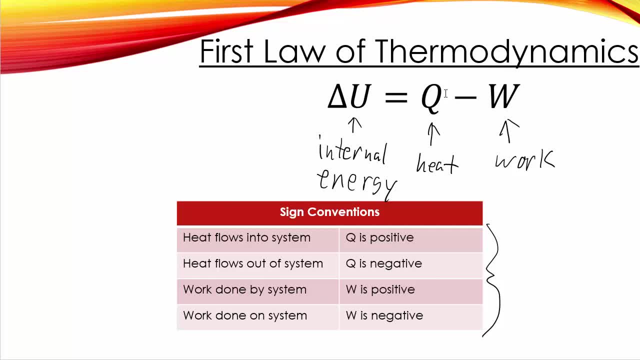 And so we would say it's positive. Now, if it's positive, we don't change the equation here. We're going to end up subtracting that work off If there's work done on the system. So something is compressing this gas. 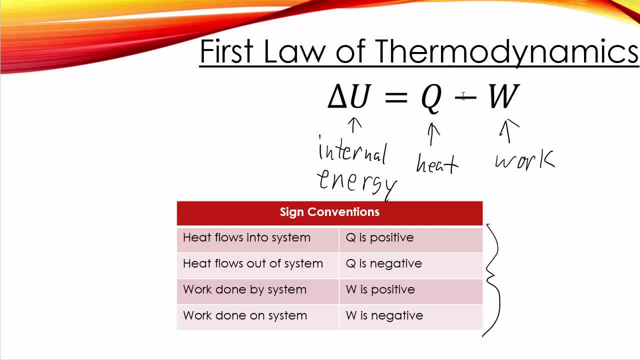 Then we would say that that is negative work And there would be two negative signs And then we would actually be adding that quantity in that situation And different texts actually reverse this. So sometimes they write their equation as Q plus W And then they just swap this sign convention. 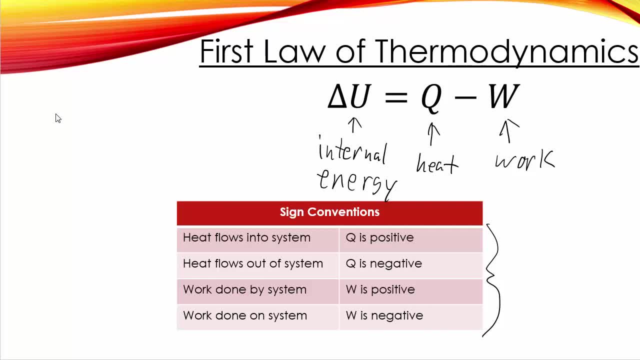 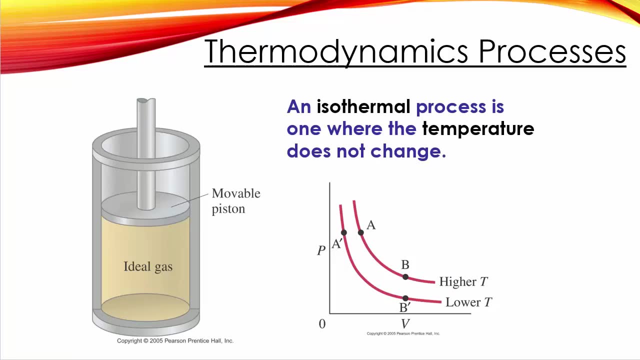 So if you ever study thermodynamics in college, be careful of that. People like to make things nice and confusing. Alright, so there are four different common thermodynamic processes that you need to be familiar with. I already showed you this slide, But this is the first one. 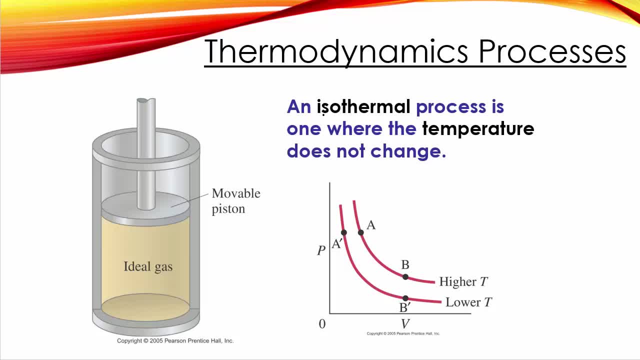 One that is called isothermal. So iso, like isolate, means something that you're not changing. So an isothermal process is one where delta T is equal to zero And the shape of an isothermal process is an inverse graph, Because in basically all of these we are assuming that the change in the number of particles is zero. 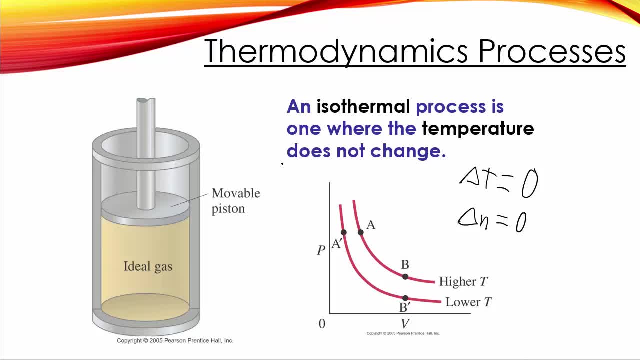 In all of these processes. So they're all either isolated or closed systems that we're analyzing. So if you're holding everything constant but P and V- we did a lab with this- then you get an inverse graph And depending on where that inverse graph lies, these ones up here are higher temperatures at a higher constant temperature. 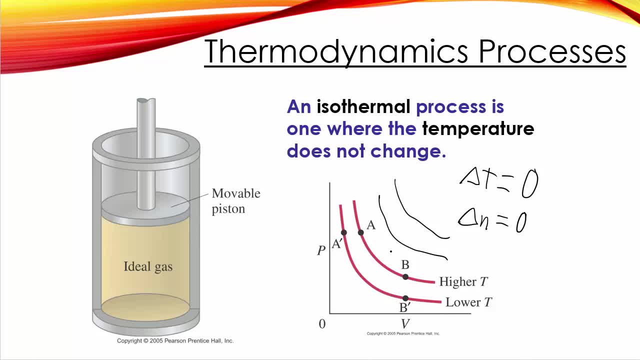 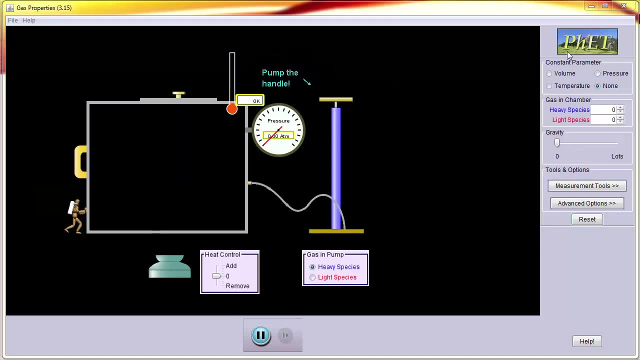 So the temperature doesn't equal zero, It's just the change in temperature is zero. An isothermal graph down here is going to be lower temperature. Okay, Now, if you look at an example of how this could actually happen, let's jump over here to a nice little FET simulation. 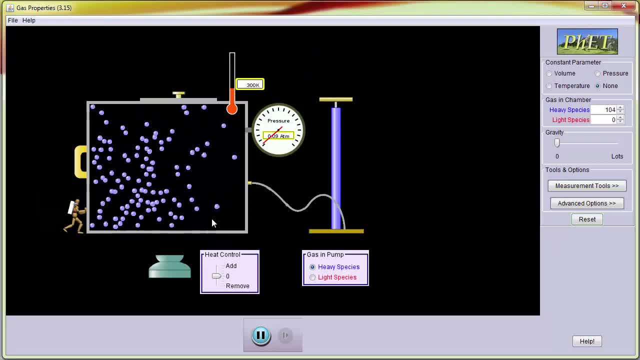 So we've got our box, Put a little bit of gas in there And over here I can choose the parameters that I want to hold constant. If I'm going to hold temperature constant, you might think: oh, that means no heat can flow. 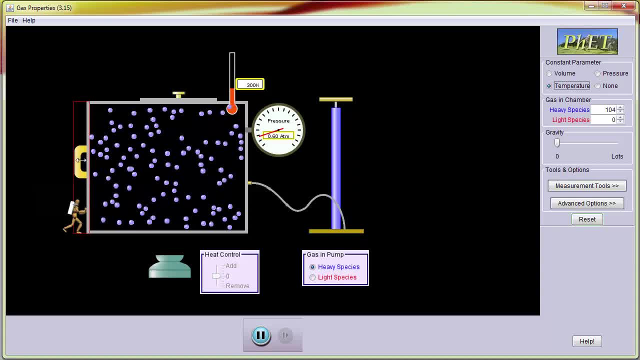 But it's actually the exact opposite, Because if I'm going to have something change, If I'm going to compress my piston or something, I change the volume, The only way to keep temperature constant. it didn't stay constant, actually, but we're bringing it back down to where it was before. 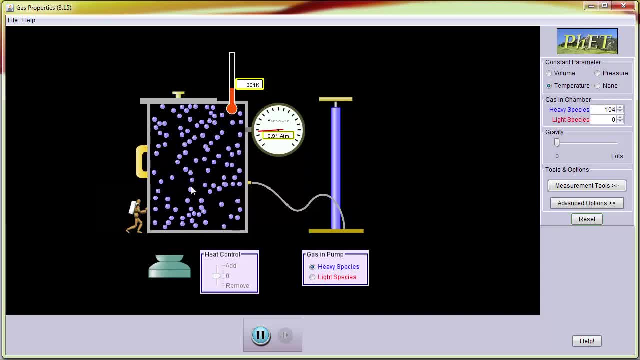 is. if you notice, there's some ice that popped out of here. So we have to have heat flow out in order to decrease our volume and not have the temperature go up. Normally, when you compress a gas, the temperature wants to rise, So we are having heat flowing into or out of the gas. 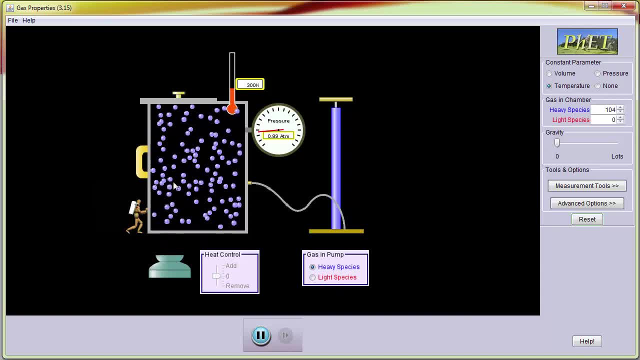 If you expand it, the opposite happens. We have to heat it up to keep it at a constant temperature, And so these are kind of ideal situations, as we like to do in physics. So in order for it to be completely isothermal, you would have to have like minuscule, tiny increases in pressure. 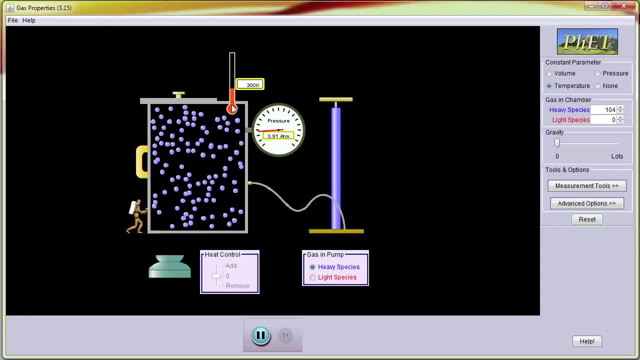 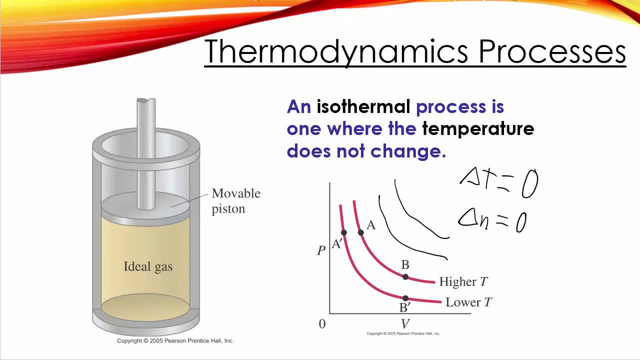 Changes in volume and changes in pressure, So slow that the temperature never had a chance to change. Okay, Now, if we think about how this affects our equations, We had the first law said: delta U equals Q minus W. In this case, delta T is 0.. 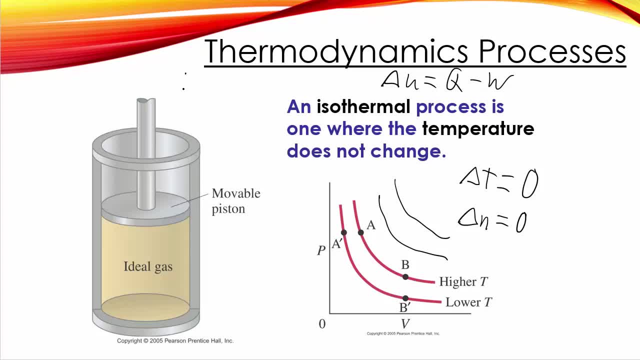 Previous to this we said that the internal energy of a gas was 3 halves big N KT or little n RT, Doesn't matter. Well, if I'm changing the temperature, then that's changing the internal energy. So you could say that delta U is 3.. 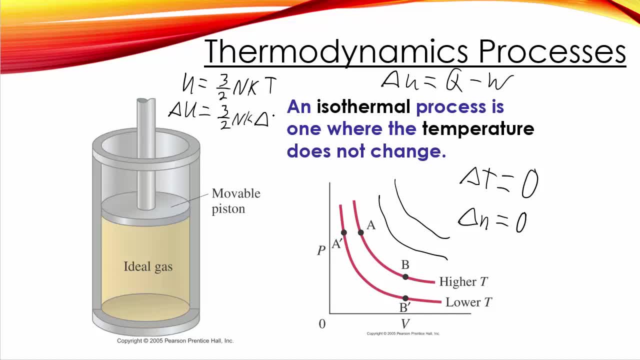 So delta U is 3 halves N, K, delta T. As long as we're holding N constant, K is always a constant. Then when delta T equals 0, that implies that delta U is also equal to 0. So if this guy over here is 0, then we have 0 equals Q minus W. 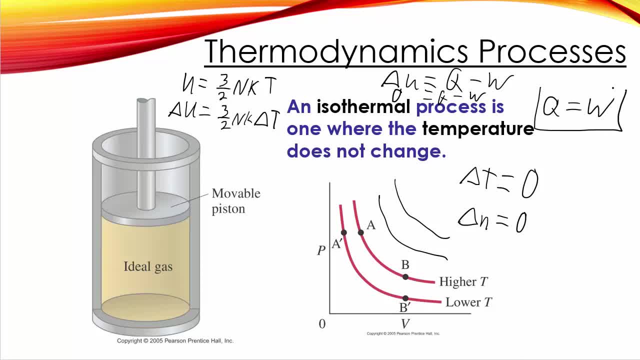 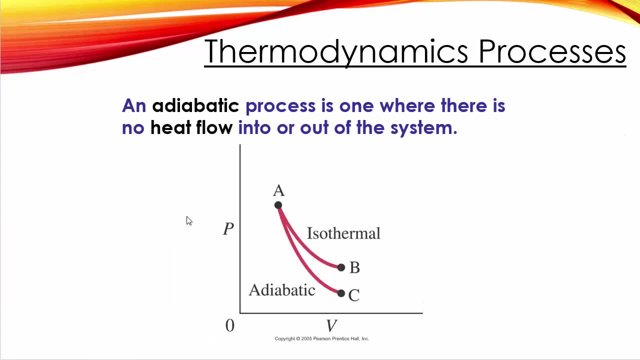 And Q equals W, So that's going to be a nice handy tool for solving problems involving thermodynamic processes. It tells you it's isothermal. You know that this relationship here is going to hold. Okay, The next type has a nice fun name. 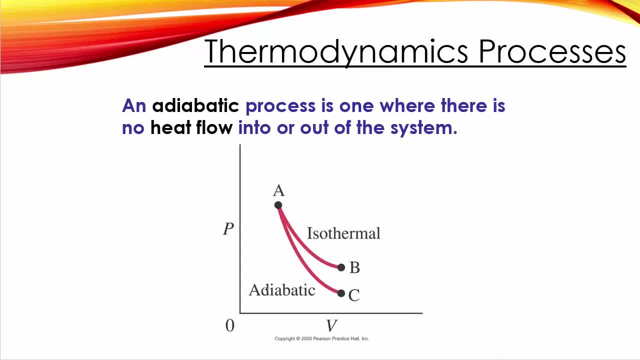 It's called an adiabatic process. I don't know the etymological roots of that word, But with an adiabatic process there is no heat flow. So by definition Q equals 0. So that means delta U equals Q minus W. 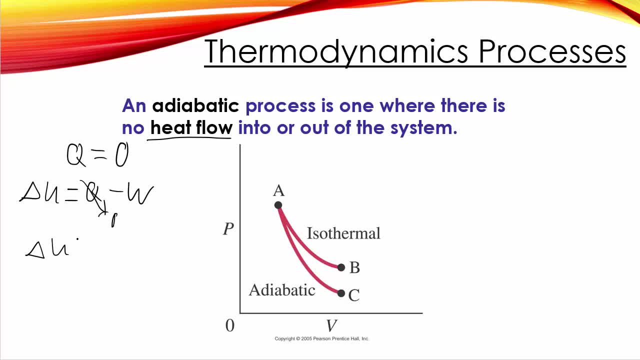 This guy goes to 0. And delta U equals W for an adiabatic process. And what an adiabatic process looks like if there's no heat flowing. that means you either have an isolated system, so heat is not allowed to flow. 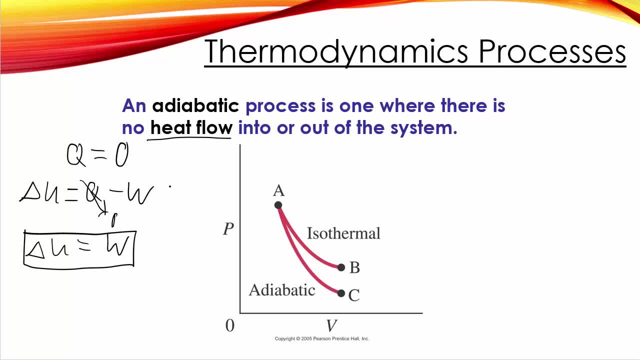 But in reality that's pretty hard to do. So what you do instead is you have a very fast process where there's not time for a significant amount of heat to flow, because it just happened really quickly. An example of that is in your car. 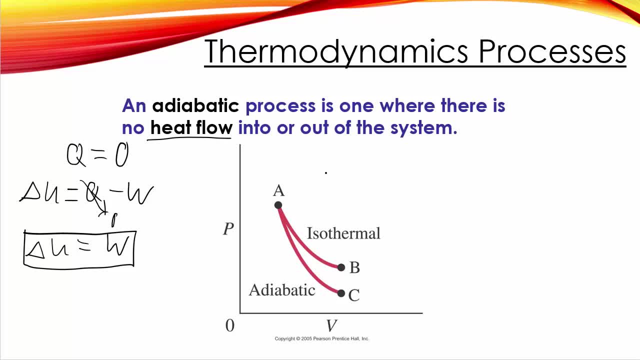 When you have an engine, when you have what's called the power stroke, where the air-fuel mixture in the cylinder explodes when it's ignited by the spark plug. that happens so quickly that no heat flows out of the cylinder, or at least very little in that short amount of time. 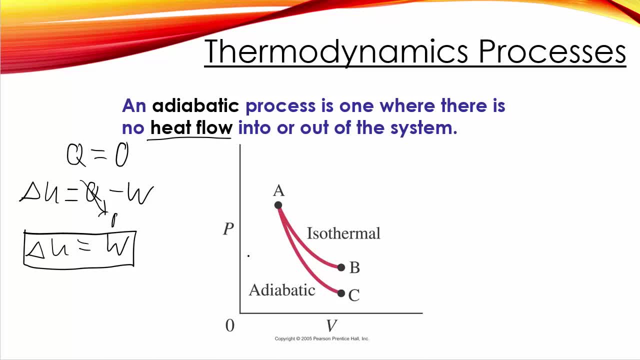 So if it expands- so here we've got a PV diagram- We're going to be using a lot of these pressure and volume If it expands so quickly that heat can't flow out or, sorry, flow in, and it's ignited at a constant temperature. 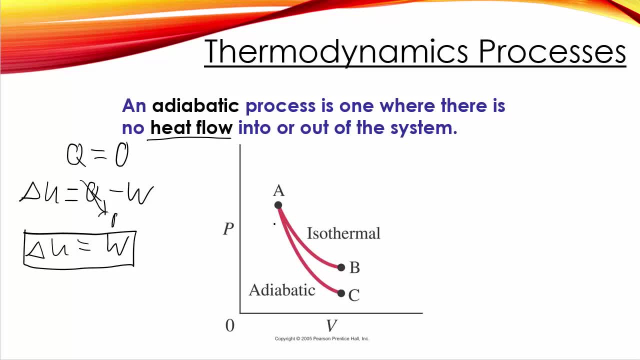 then it's got to cool off. So if we think about this line- here is our isothermal line- and if we've got a bunch of isothermal lines, like I mentioned earlier, representing different temperatures, if we're down here on this isothermal line, 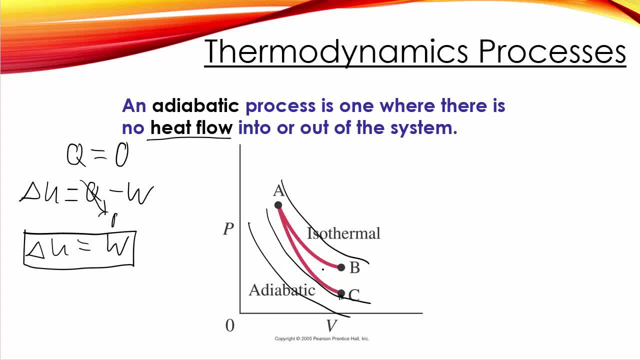 we didn't follow that line, but that's where we ended up. then we had to cool off because the volume increased, which tends to make things cool off unless you have time to absorb some heat. But by definition we're saying you can't absorb heat. 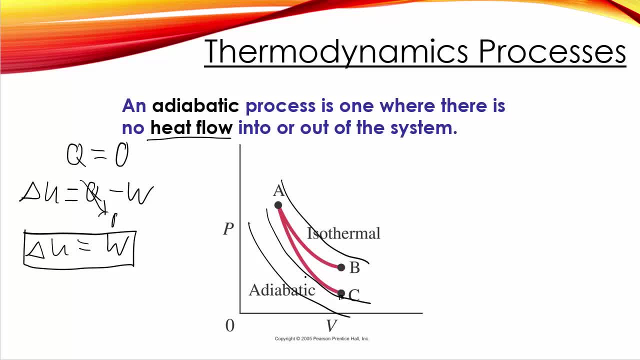 or it has to cool off. going this way: if it's adiabatic, It has to heat up. going that way: if it's adiabatic, because you don't have time for the heat to flow out, going that way as well. 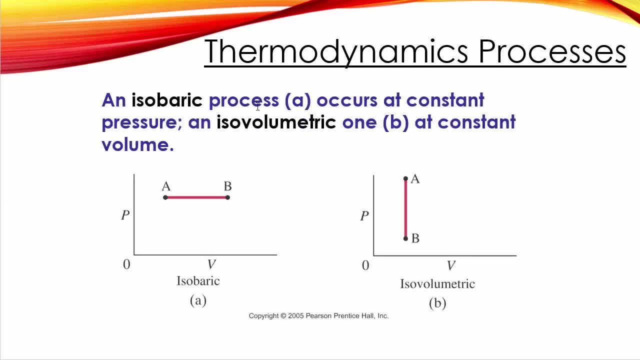 Okay, two more of these guys. We have isobaric, which is a little easier to remember, So baric. if you think like barometric pressure, then isobaric is constant pressure. Isovolumetric has the word volume right there in the middle. 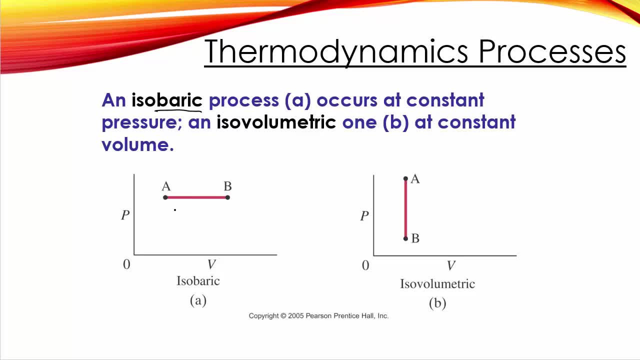 so that means constant volume. So constant pressure is just going to be a horizontal line on a pressure-volume diagram. As you change the pressure- sorry- as you change the volume, the pressure remains constant Here, as you change the pressure, the volume remains constant. okay. 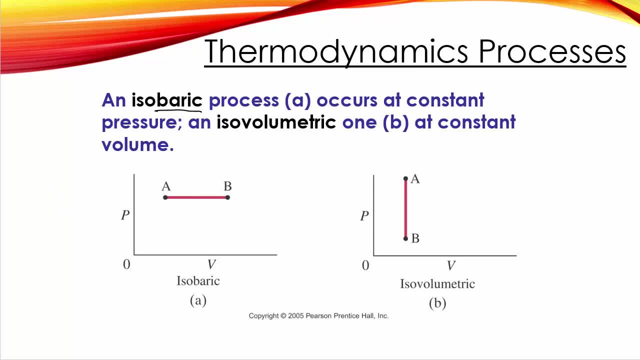 And these have different implications as well for our calculations. So let me find my pen. The pressure times, the change in volume, is actually equal to the work done. Pressure times volume gives you an energy, so pressure times change in volume is a change in energy. 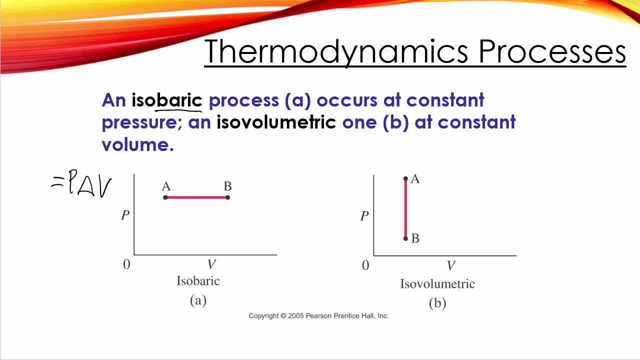 And my W's having problems. And change in energy is defined as work And if you're going this way your change in volume is positive. so we'd say there's positive work done. If you're going the other way, then we would say your change in volume is negative. 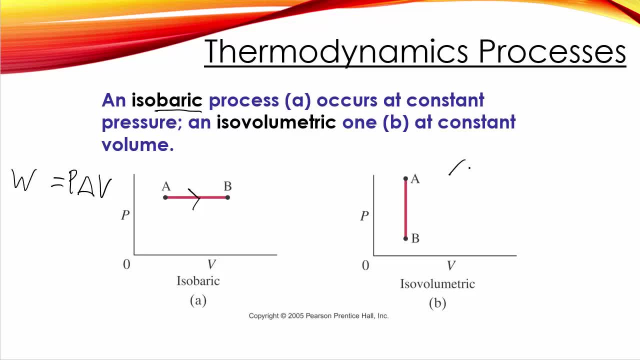 so you would have negative work Here. delta V is zero, So that means the work done is zero whenever you have isovolumetric. So back to our first law equation: delta U equals Q minus W Over here we can just say that delta U equals Q. 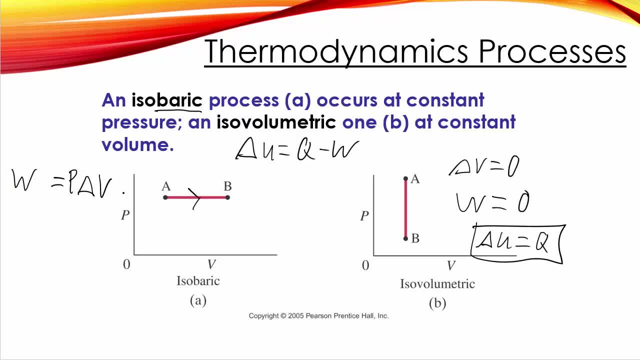 And over here nothing really cancels out. You can still have Q changing Q, that's nonzero, So we have Q. oops, didn't mean to write W and delta U equals Q minus P, delta V. Okay, So if we kind of summarize what's going on with all of these things, 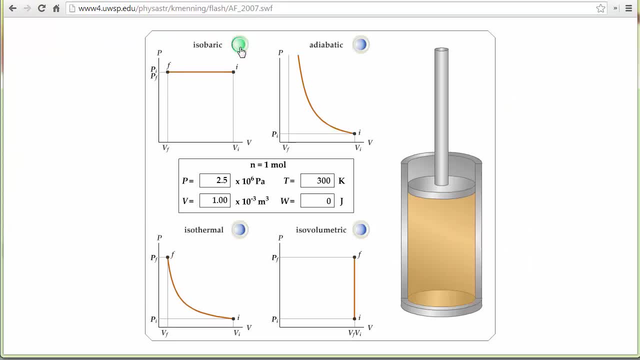 if you imagine a piston going up or down, the animation isn't all that useful. it just kind of repeats. But if you pay attention to what's going on with these values here, it's kind of useful. So isobaric, that's constant pressure, and we're going to animate this. 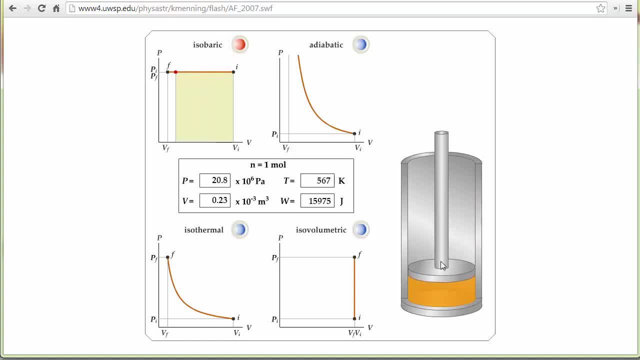 So if I'm compressing a gas but I don't want the pressure to go up, I have to have the temperature to go down right, Because as temperature goes down, then pressure goes down. So if I'm holding pressure constant while compressing, 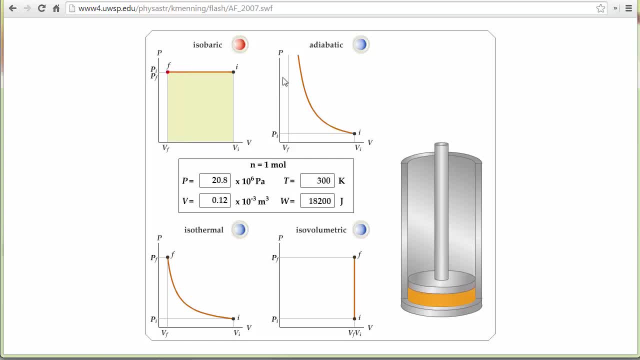 temperature has to go down as well as the volume Adiabatic. here I'm compressing it and I'm doing it really quickly, even though the animation isn't showing that. If that happens, I don't have time to let any heat flow out. 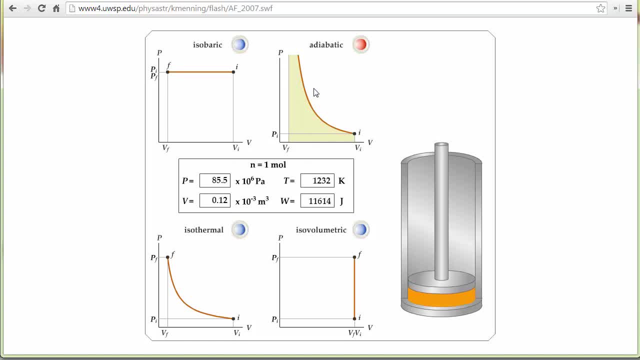 so the temperature is going to go up. Essentially, you have all three things changing at once in an adiabatic expansion or compression. So the pressure goes up, volume goes down, temperature goes up as well. You always have to have a temperature change on an adiabatic process. 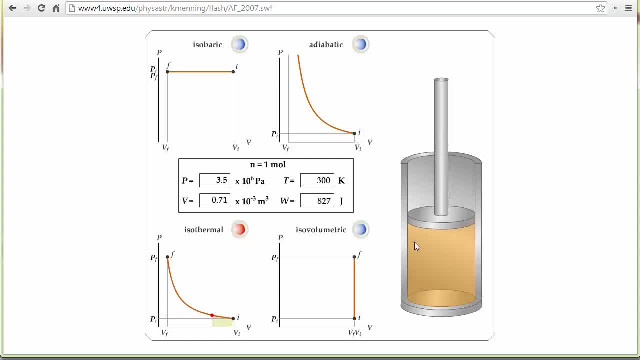 Okay, isothermal. here we're holding temperature constant and this would be kind of opposite of adiabatic. instead of being really quick, In reality this would be an incredibly slow process so that you would allow enough heat flow in or out. 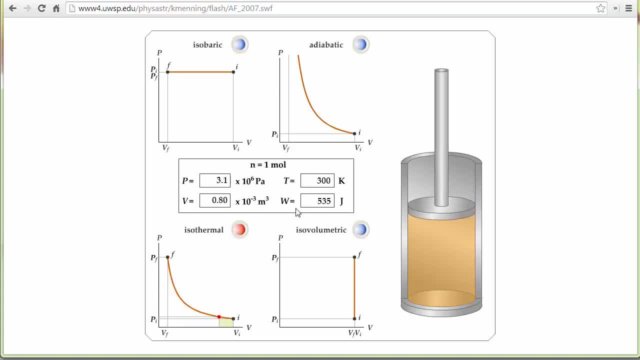 to hold that temperature constant. In this case, you would want heat flowing out in order to hold that temperature constant. Pressure can still go up. volume goes down, obviously because you're compressing and that means there's work being done on it. 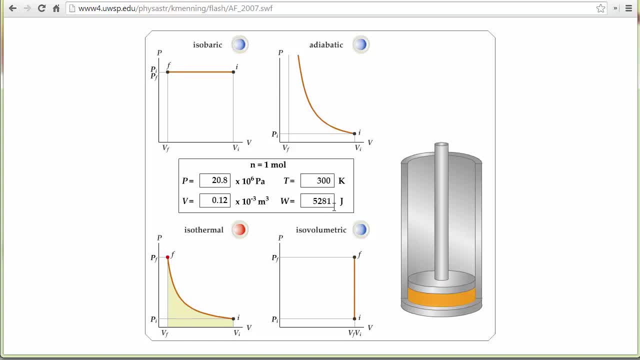 which, yeah, that would be positive in this case. Okay, isovolumetric animation is pretty exciting. You're holding the volume constant. so if you want to change pressure without changing the volume, the only way to do that is to let some heat flow in. 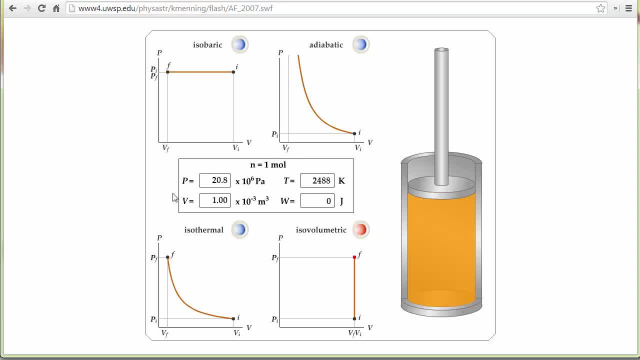 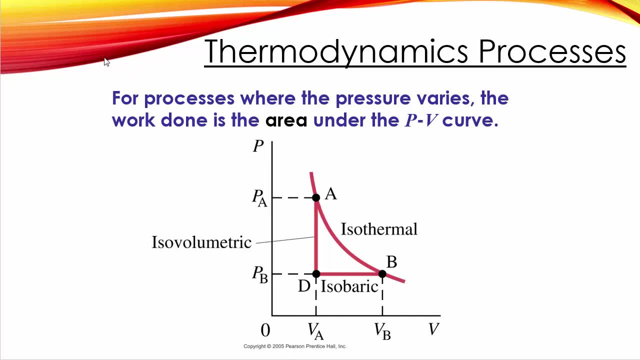 and that results in a temperature change. Now, a lot of times we will combine these different processes into a cycle. Usually there's a direction to these things, so we'll have arrows. We might say we started at A and we had an isothermal expansion. 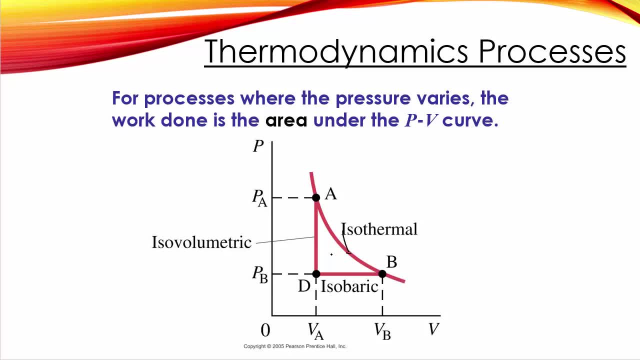 By expansion we mean volume increased. So we would say we went this way along our isothermal line, Then we would have an isobaric compression, because then our volume went down, We compressed it and we did isobaric there. 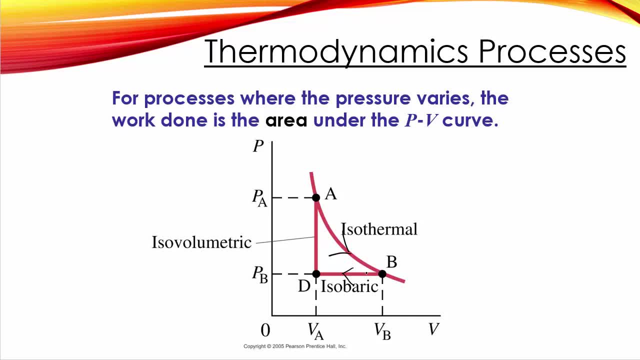 so we let more heat flow out, And then we did an isovolumetric pressure increase. We pressurized it isovolumetrically. So as you go around that curve, that would be your cycle of your thermodynamic process. Now in our equations we're pretty much only going to calculate the work done. 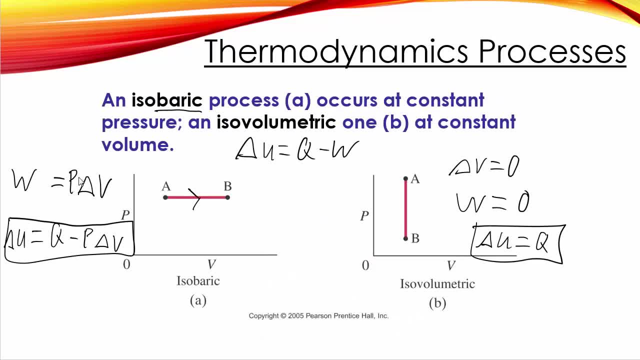 when we've got an isobaric process: P delta V. Otherwise we would need an integral and this class isn't calculus-based. Basically, you've got work is the integral of P- dV, but we're not going to be dealing with that. 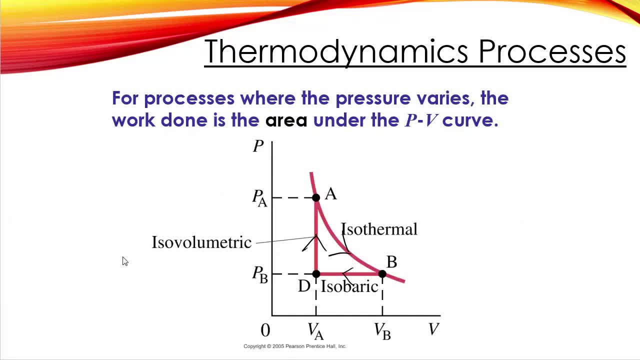 But it is still true that the area under the curve on a P-V graph is the work done, And I do want you to be familiar with that kind of concept. So what's going on here is, during this isobaric process, the work done is this area right here. 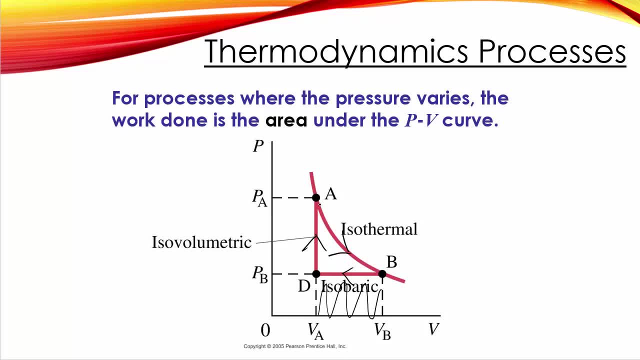 but it's going to be negative. And then during the isovolumetric there's no work done because there's no area under that line- Isothermal. here there's going to be positive work. Let me grab a different color here. 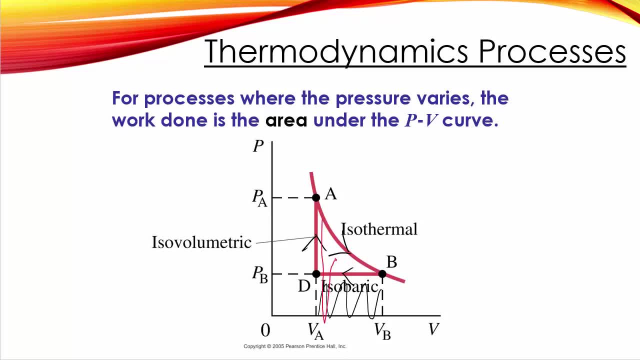 And it's not just the area inside, but it's the entire area here. Okay, so the red would be some positive work, Positive work, The black part would be negative work, And if you wanted to find the network for the entire cycle, 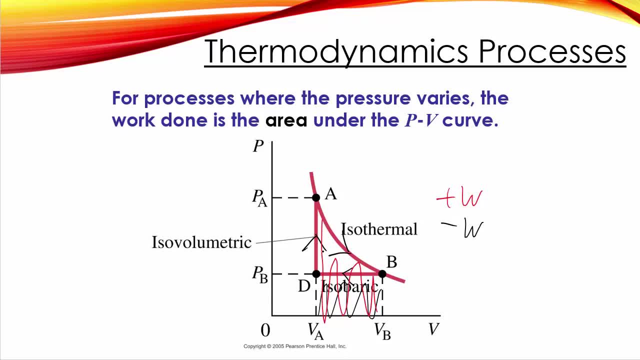 well, it would be the red minus the black. So let's grab green here or something. So it would just be the area enclosed by the cycle is going to be the network done going around the cycle And that's going to be useful. 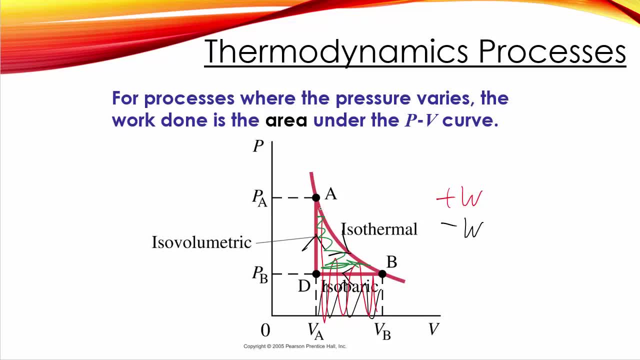 Conceptually for some of our calculations. We're not going to be able to calculate this directly, but if we know the total work and we find the work done here, then we could find the work done in that isothermal process or something along those lines. 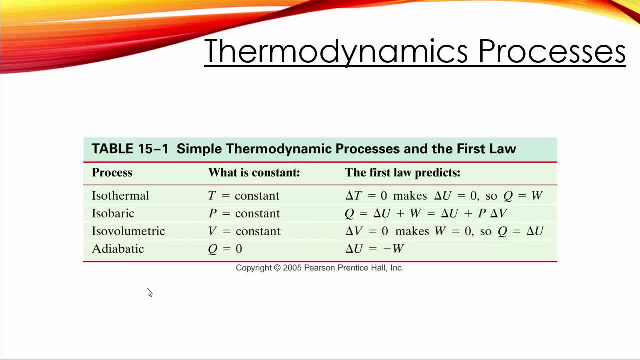 Okay, in case you didn't take notes the first time, here is a great little summary- And this is in your book somewhere- Of all the implications for our calculations for all these different processes. So isothermal constant temperature: delta T is zero. 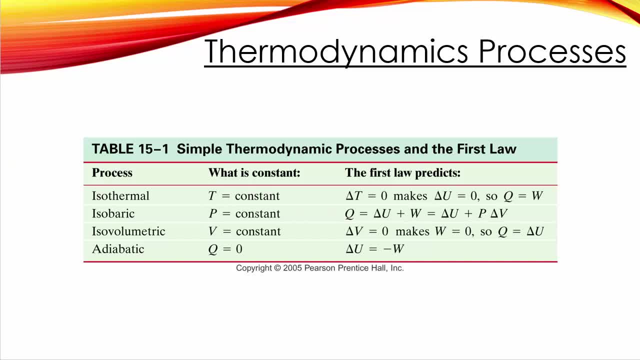 so delta U is zero. so Q equals W. P is constant. so all we really change is we define W as P delta V Isovolumetric. that means that delta V is zero, which makes work zero. so Q is equal to delta U. 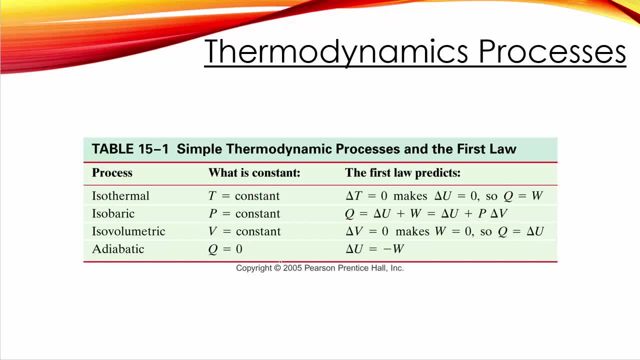 And adiabatic. by definition, Q is equal to zero, so we get delta. U equals W. Probably want these written down somewhere for future use. Okay, see you next time. 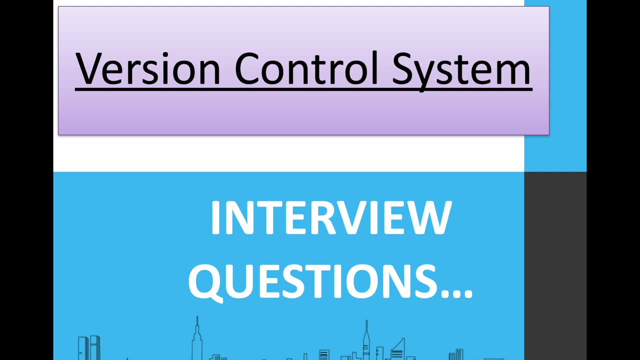 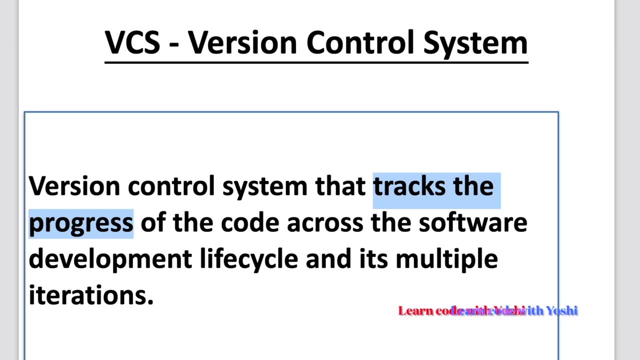 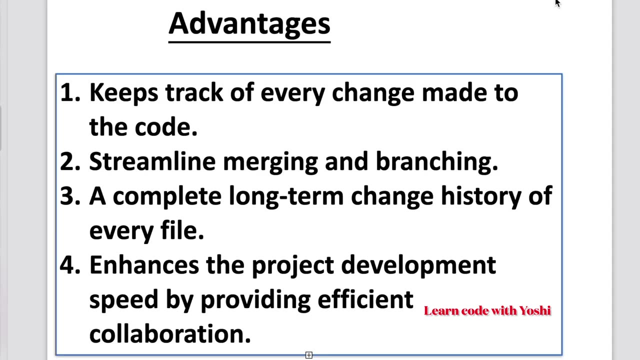 Hello all. let's briefly talk about what is version control system and benefits of using these tools. Version control system is a system that tracks the progress of the code across the software development lifecycle and its iterations. The advantages are: it helps to keep track of every change made to the code, like which developer did what and what time it has done those kind of details. 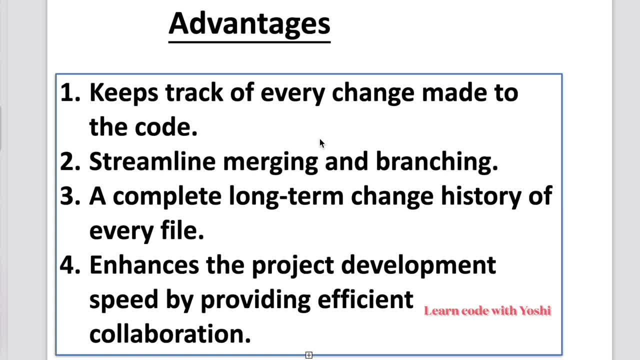 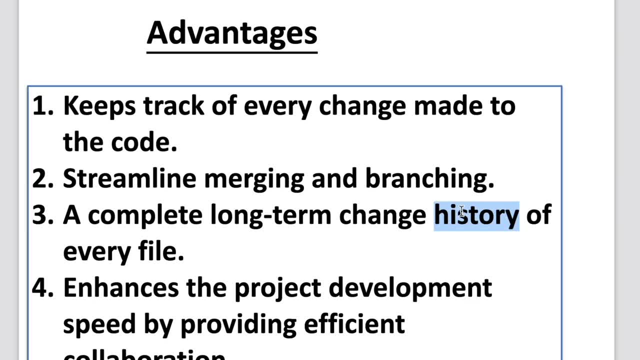 It also helps to streamline the merging and branching. I'll be talking more about what is branch and what is merge- those kind of commits- in the future videos. With the help of these tools, we can also make a complete long-term change history of every file. 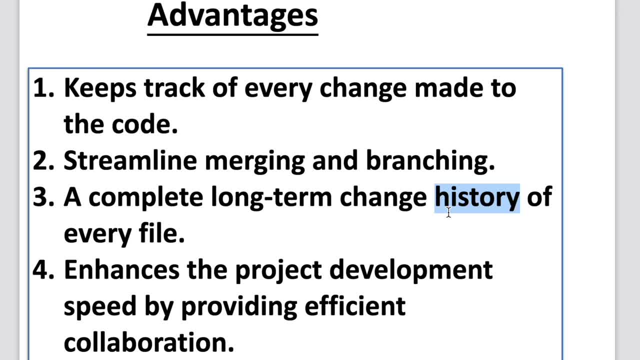 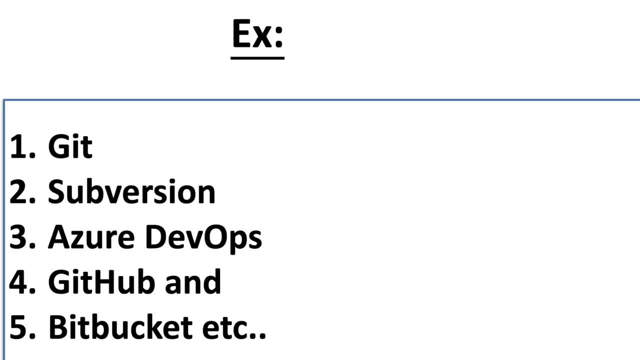 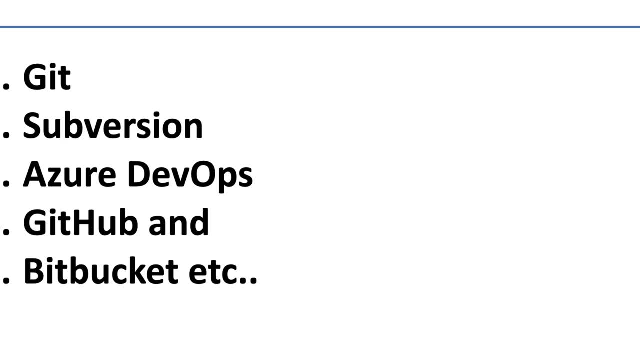 And also, it's obvious, right. it enhances the project development speed by providing efficient collaboration. There are few popular version control tools like git subversion, azure devops, git hub and bitbucket. In real time, the companies might opt anything whatever comfortable for them.